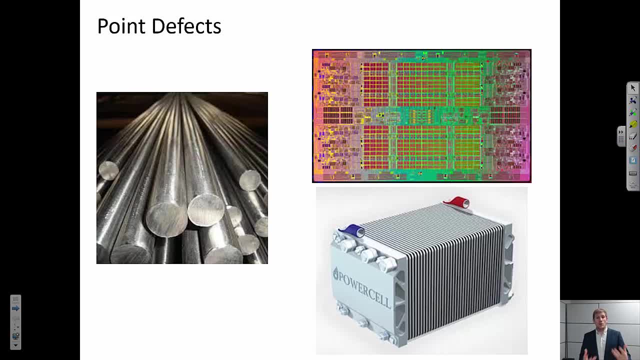 but you can control the number of charge carriers and what type of charge carriers they are in a system by controlled doping of different electron donors or acceptors in a system. Finally, we might want to control the motion of point defects throughout a material. So this is the case in a fuel cell where we need certain atoms to migrate. 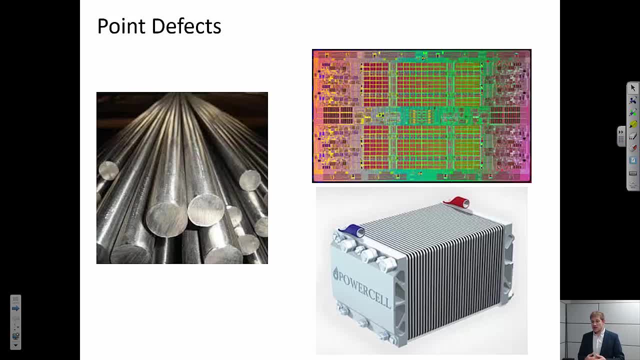 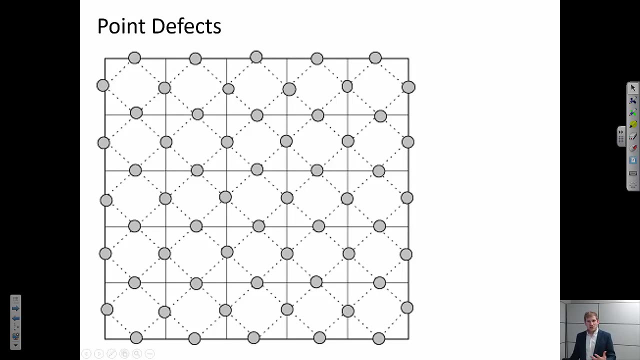 from one side of a material to another side. So we want to make it easy for there to be vacant sites for these atoms to move along in. OK, so what are some of the different kinds of point defects that we might see? We're going to first consider the metallic systems, And there are three basic kinds of defects that we're going to talk about. 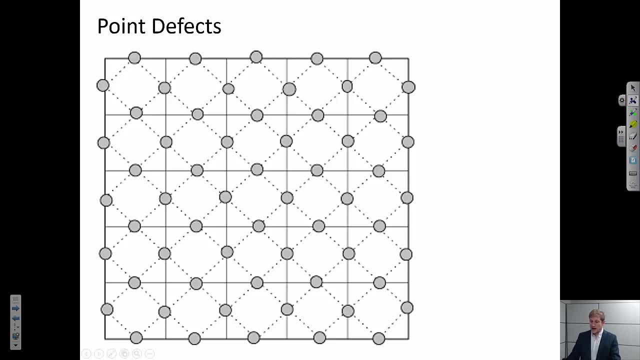 The first is the metallic system, which is the one that we're going to talk about today. The first is called a vacancy. So this is our lattice here: If one of these atoms was missing, it's not there. That is what we call a vacancy. 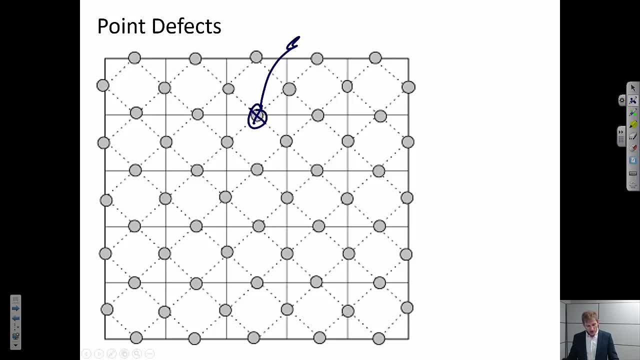 Now I'm going to show you the notation for these different kinds of defects as well. So if we have a vacancy, we symbolize that V for vacancy. Then we say what the atom was that is missing. So it was on an aluminum site, say, 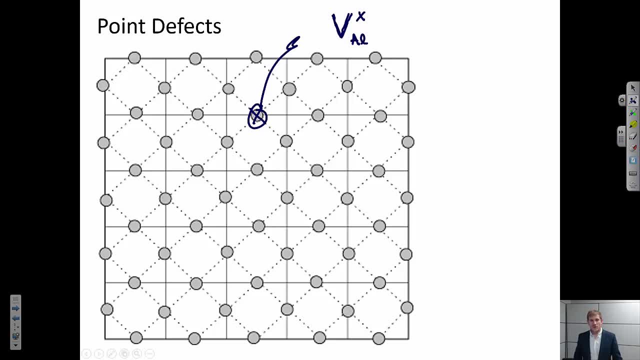 So this aluminum site is gone And then we give a symbol that refers to the charge of this point defect. So in this case aluminum vacancy and aluminum lattice is a neutral charge. So we put an X there. So vacancy is the first type. 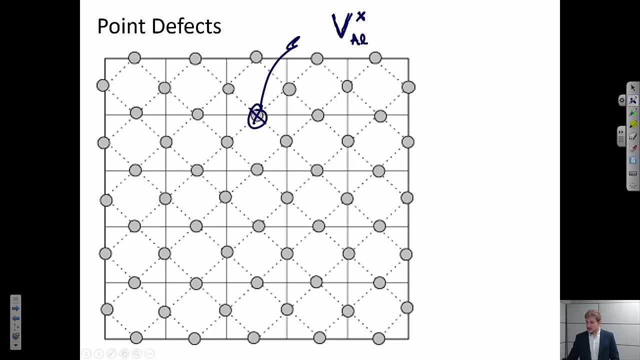 The second type would be an interstitial, And that is if we have some other atom sitting in a site in this lattice that is not normally occupied. So let's say, for example, this is still an aluminum atom. I'll say aluminum there. 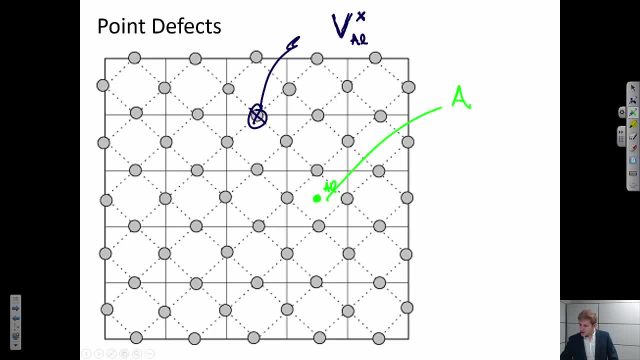 We would notate this. So this is now an aluminum atom And it's on an interstitial site. That's what the I means. And again, it's a neutral charge. So we give a neutral sign. That's the X symbol up there. 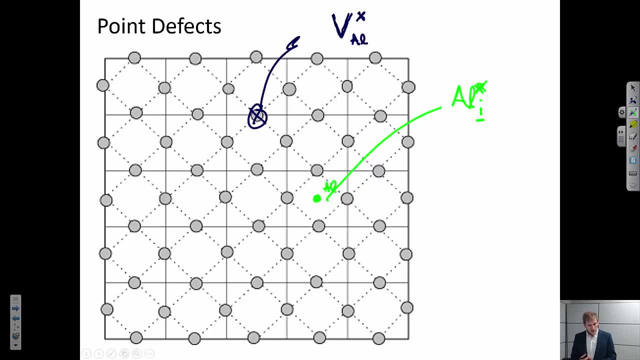 The third kind of point defect we would see would be a substitution. So again, let's say this is a lattice of aluminum atoms, But this atom here is not aluminum. Let's say this is copper. So the notation for this is going to be written as such. 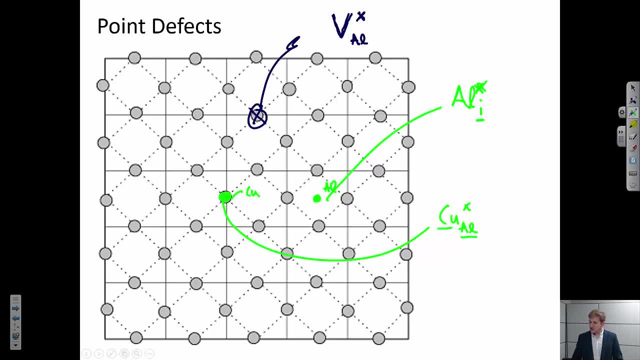 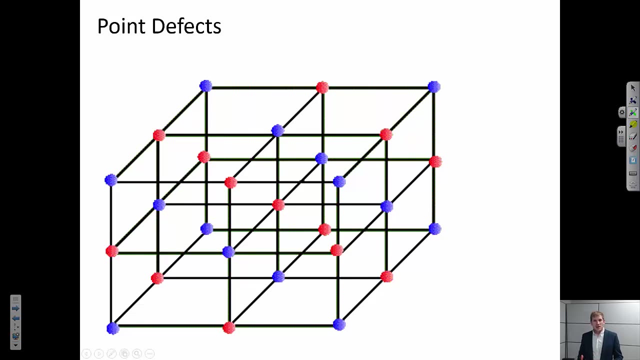 So again, a copper atom is sitting on an aluminum site And the net charge is neutral. So these are the three different kinds of vacancies, Of point defects. We have vacancies, we have interstitials and we have substitutions. Okay, next we're going to think about ceramic or ionic compounds. 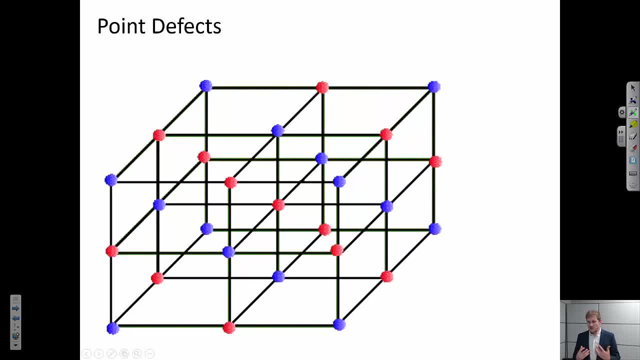 And there are additional things that we have to consider in these cases, And that's just because an ionic compound has positively charged ions and negatively charged ions. So let's say, each of these blue is a cation and each of the red is an anion. 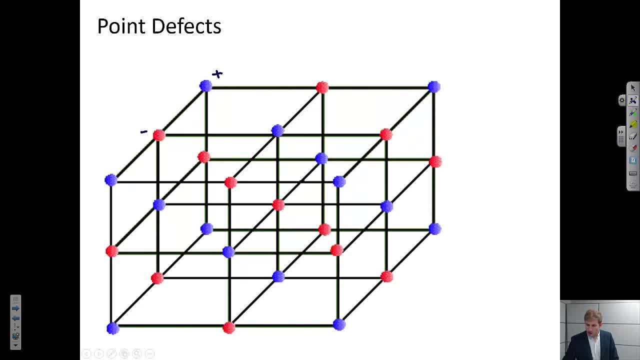 And for the purpose of this, let's say these blue are magnesium, So it's actually plus two, And the red are oxygen, so it's minus two. So in the ionic case we can't simply have a vacancy of one of these atoms. 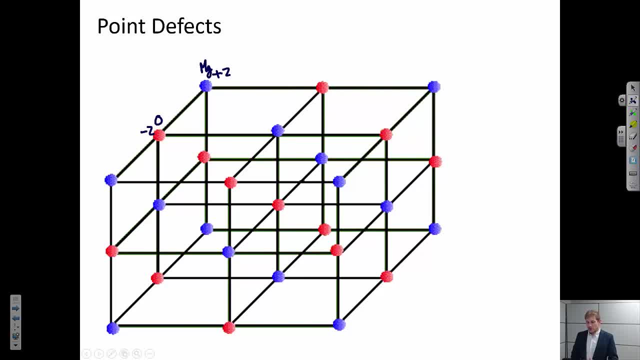 Because that would lead to a charge imbalance in the system. Similarly, we can't just have a substitution of one other charged species in the lattice, Because that would also lead to a charge imbalance. So the rule is that when we're dealing with ionic compounds, we always need to maintain charge balance. 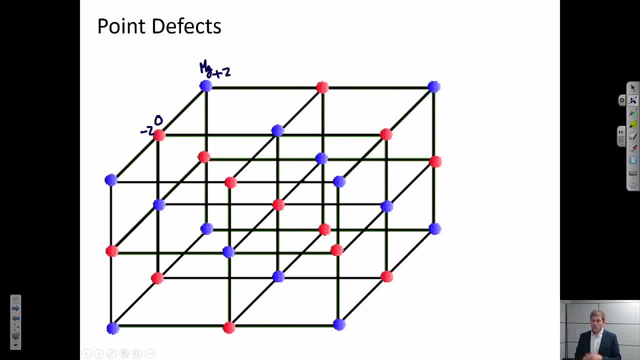 Because of that. there are two special kinds of point defects that we see very frequently in ionic systems. The first are called Schottky defects, And this is when we have a paired vacancy. So let's say, both this magnesium and this oxygen atom are missing. 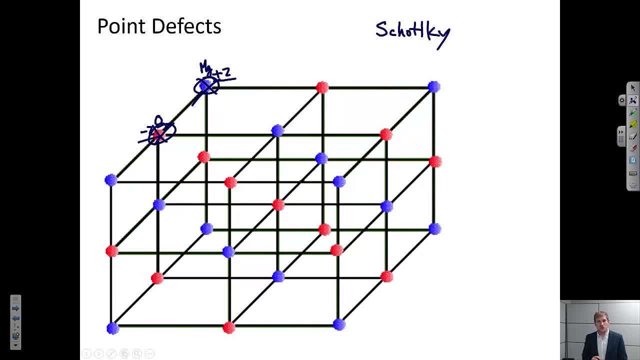 We're missing a plus two charge and we're missing a minus two charge, So we have maintained charge balance, The notation for this. I'm going to write it first and then I'll explain what it means. Okay, so I've written it like a reaction. 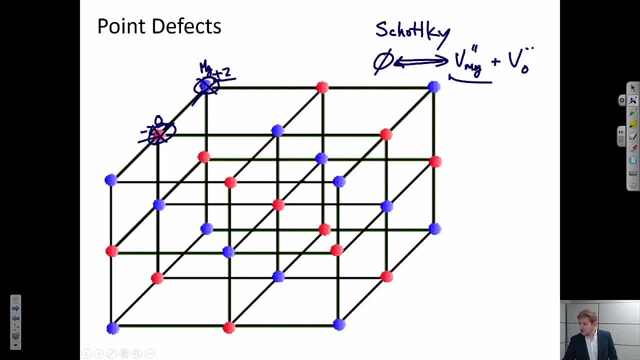 So initially we have the pure lattice, But we went to the case where we have a Vacancy of a magnesium cation and a vacancy of an oxygen anion. Now you'll notice that I didn't put an x up here, Because both of these are charged species. 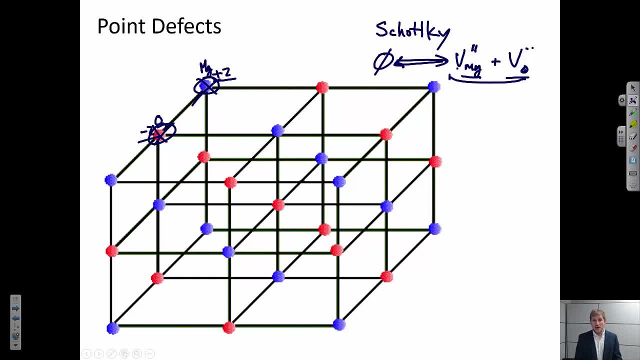 Magnesium has a plus two charge. So if we have a magnesium vacancy that means we have a negative two charge, Because that positive two that is usually there is not there. So negative two charge is written by two dashes up here. Similarly, a vacancy of an oxygen would have two positives. 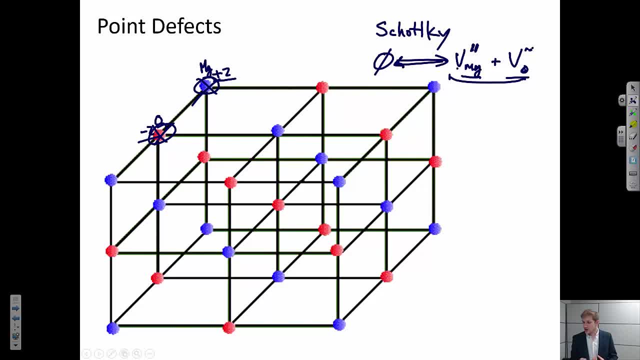 And a positive charge. so we notate that by two dots up here. So this would be a single magnesium vacancy, a single oxygen vacancy. But again the Schottky defect is where we have the case of the paired vacancies. Now there's another way that we can maintain charge balance. 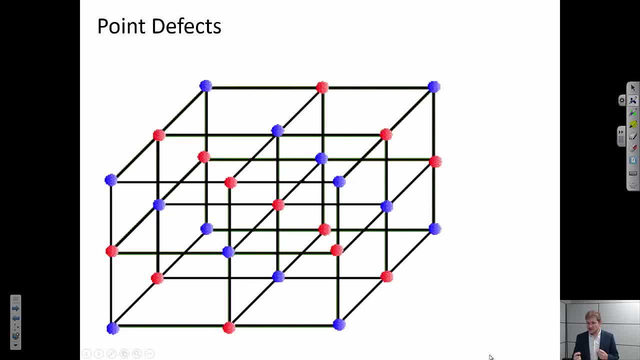 And that's, instead of removing a positive and removing a negative species, we could remove a positive species but then put it somewhere else in the lattice. So again, let's say these blue are our magnesiums. So let's say this magnesium atom leaves its normal site. 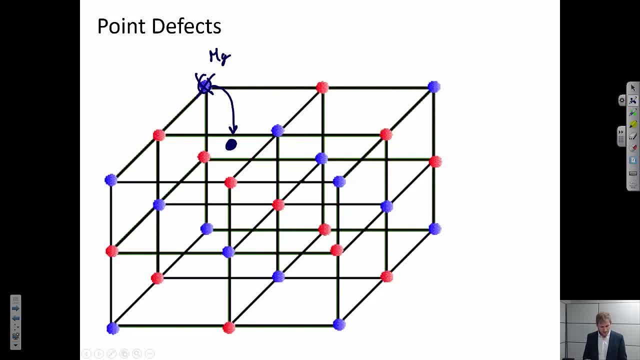 and comes to sit here in an interstitial site. So this is what we call a Frenkel defect. I'm going to again I'll write out what the reaction looks like and then I'll explain the notation. So originally we had a magnesium on a magnesium site. 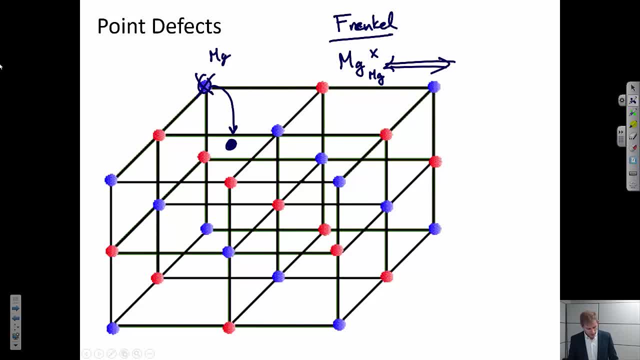 And that was not charged. And again, I write it as if it were a chemical reaction. I now have a vacancy on the magnesium site. So magnesium is two plus, The magnesium vacancy would be two minus, And they have a magnesium on an interstitial site. 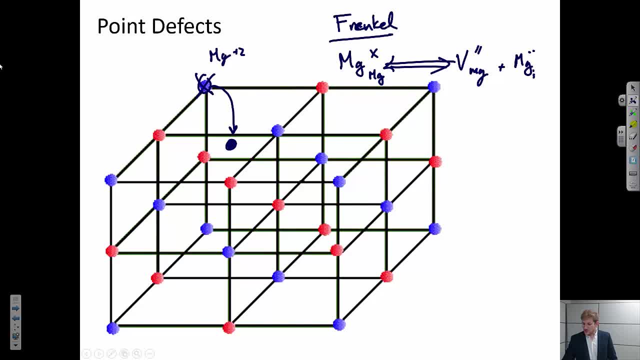 So the magnesium now is two plus And because it's on an interstitial site we say that has two plus charge. So one of the things you note you can see with this notation is that the charge on both sides of the reaction is equal.